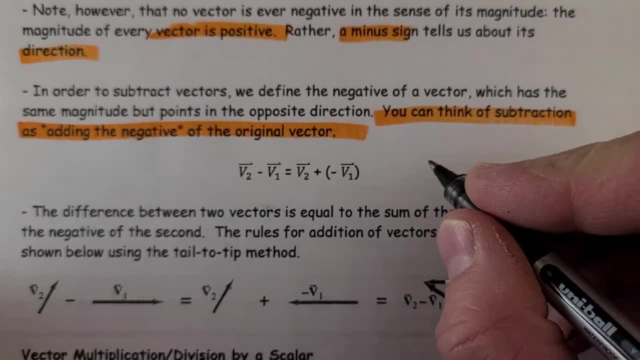 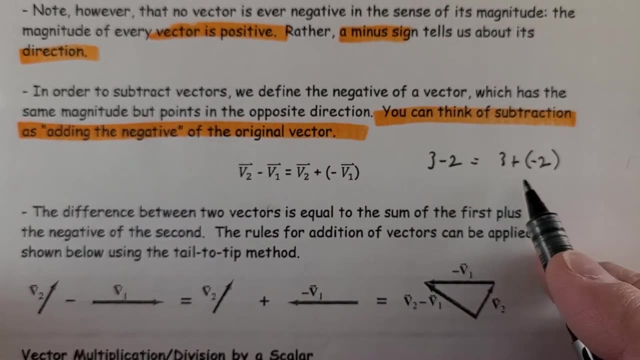 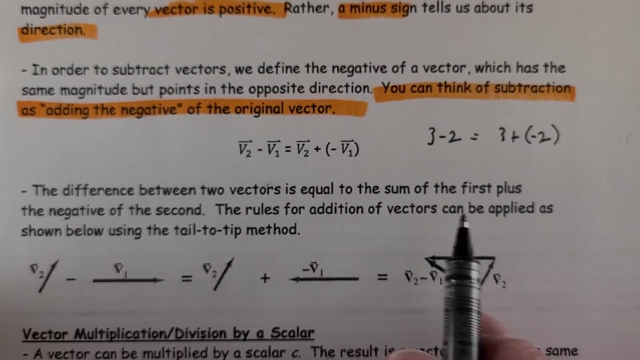 we can think of that as vector V2 plus the negative of V1. So if I was looking at regular subtraction, we can think of it as adding the opposite. Three plus a negative. two is the same thing as three subtract two. The difference between two vectors is equal to the sum of the first vector. 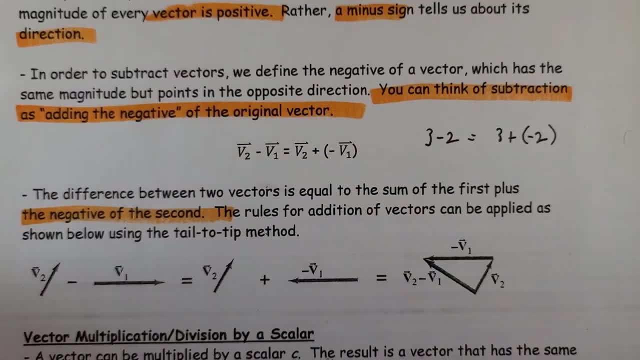 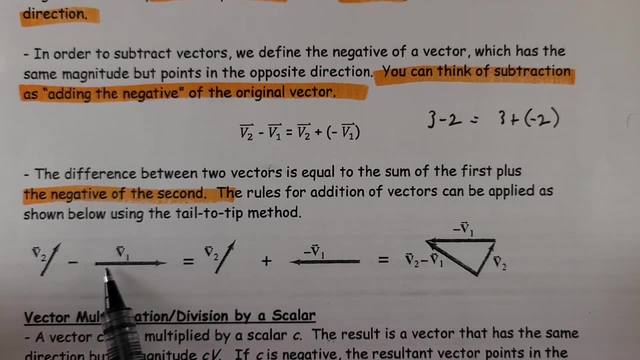 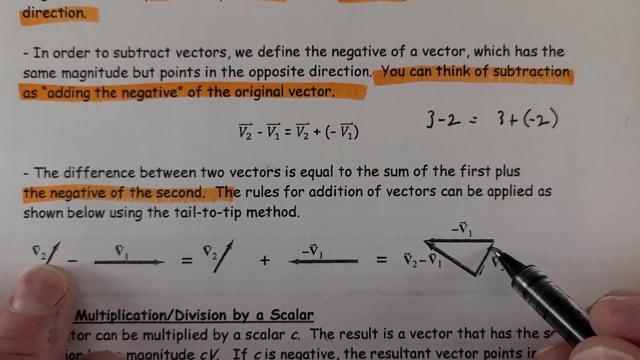 plus the negative of the second. So, for example, if we looked here, if we had V2 subtract V1, it'd be V2 plus the negative of V2. So you can see it's pointing in the opposite direction. So our V2, here it is here, plus the V1 negative. 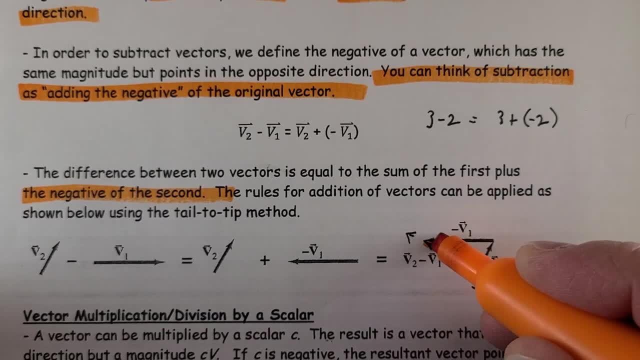 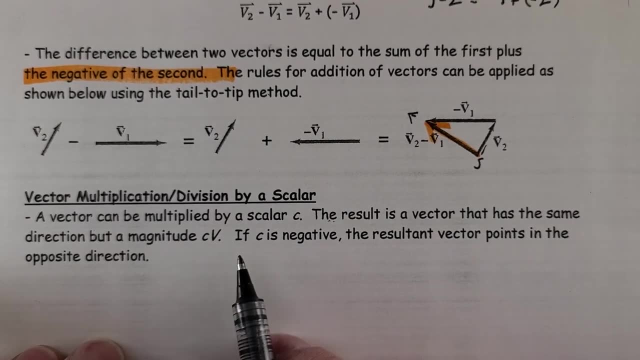 So start to finish, and there it would be right there. So again, it's vector addition, but it's adding a negative. That's it. Vector multiplication or division by a scalar. Vector can be multiplied by a scalar. We can call it c. 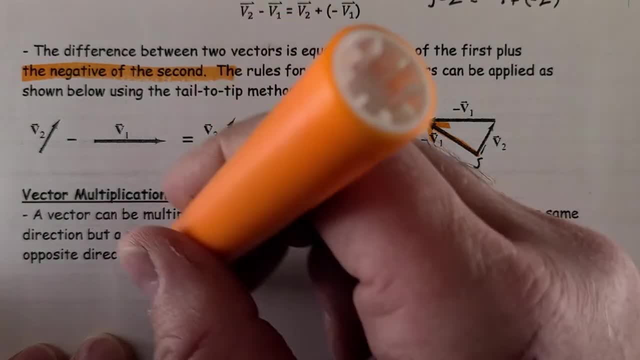 The result of the vector has the same direction this time, So we can call it c. The result of the vector has the same direction this time, So we can call it c. The result of the vector has the same direction this time, So we can call it c. The result of the vector has the same direction this time. 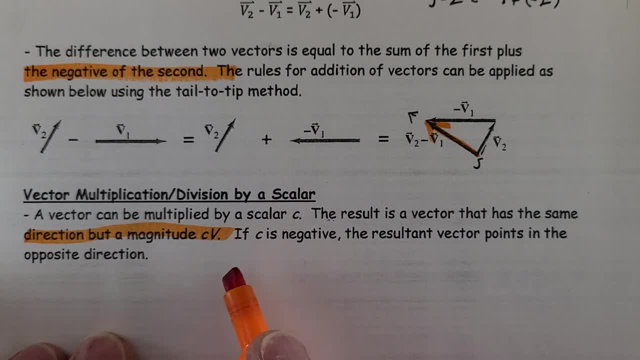 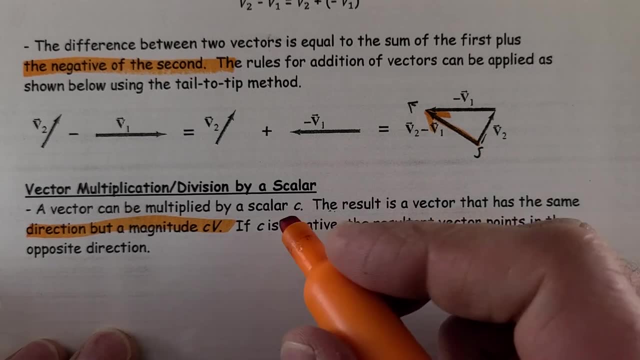 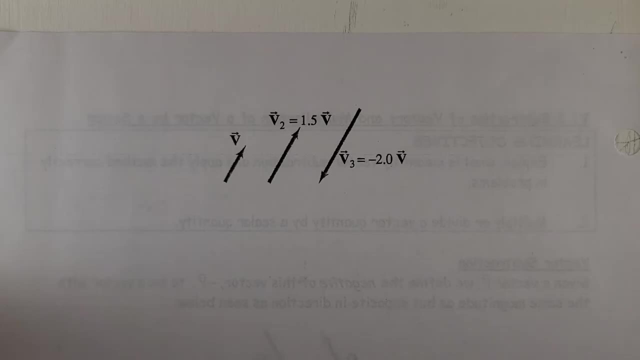 But its magnitude is going to be affected by c multiplied by V, or multiplied by a half, or divided by two, et cetera. Only if c is negative, then I change it to the opposite direction. Only if c is negative, then I change it to the opposite direction. 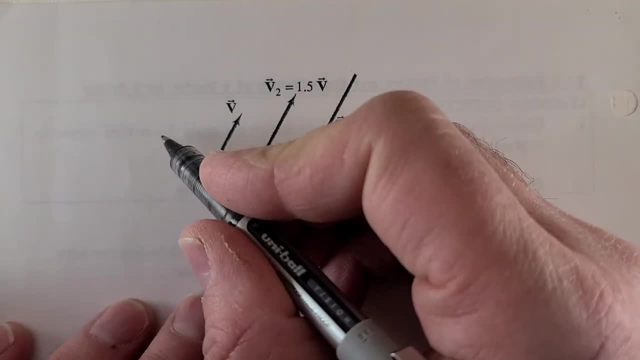 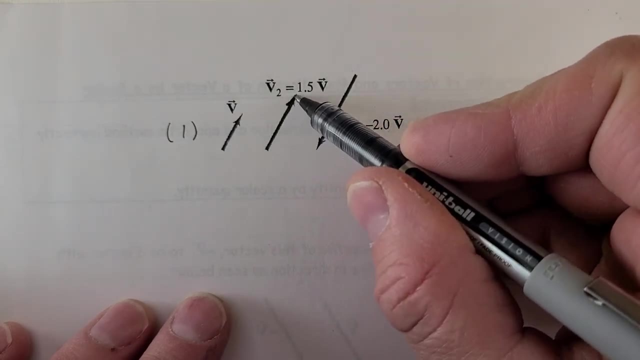 So, for example, if I look at the flip side, if I have a vector V- let's say vector V just happens to be one unit, then 1.5 times that would be well 1.5.. If I was to take the negative 2 times V. 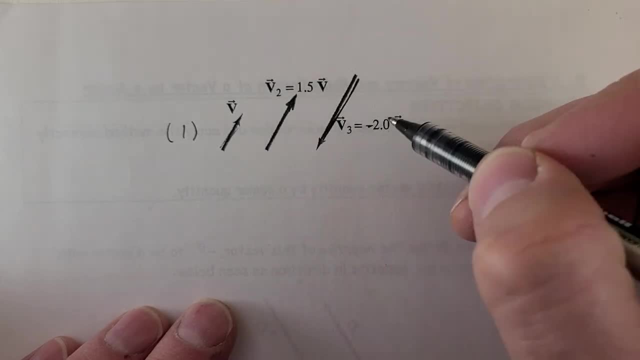 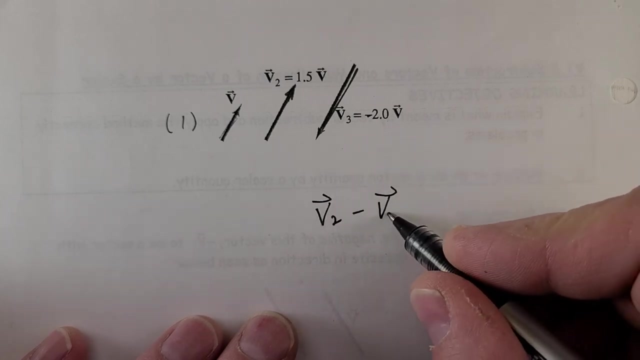 it'd be twice as long, but opposite direction. So if this is north 25 east, it'd be south 25 east. That's it. That's how you handle that. So just change. If I have vector V2 minus vector V1,. 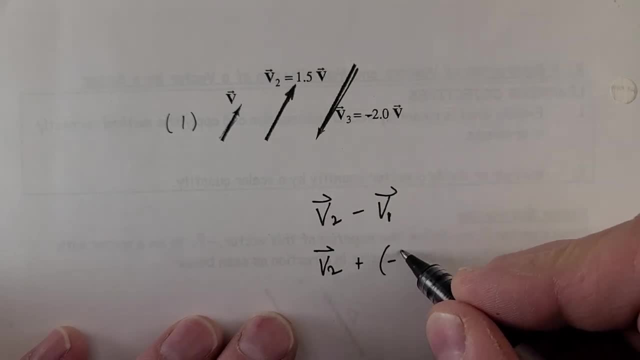 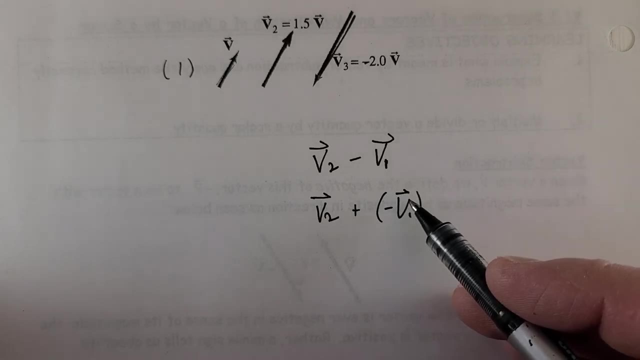 again. think of it as vector V2 plus the negative of V1, the opposite. So all you have to do is just change the direction of this vector that we are subtracting and we can add the opposite there. All right, So that was simple. 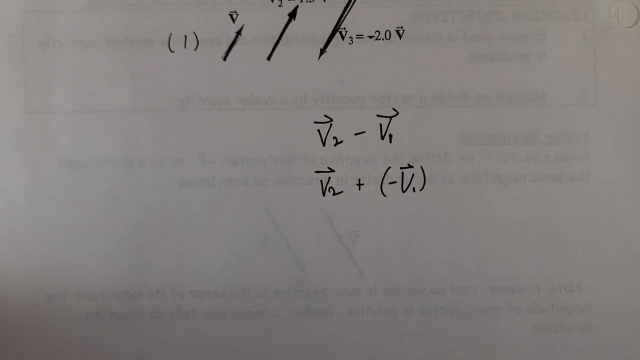 We should be able to do the assignment for that now, after that quick part. All right, We'll see you again.